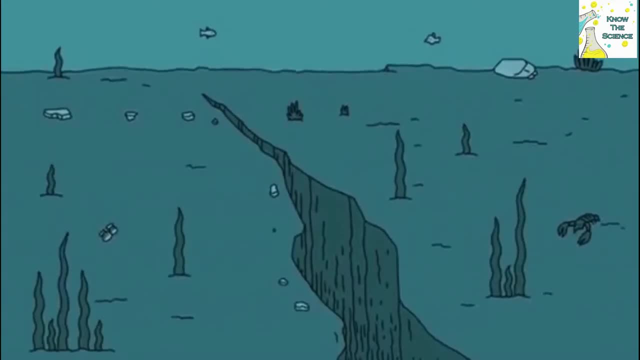 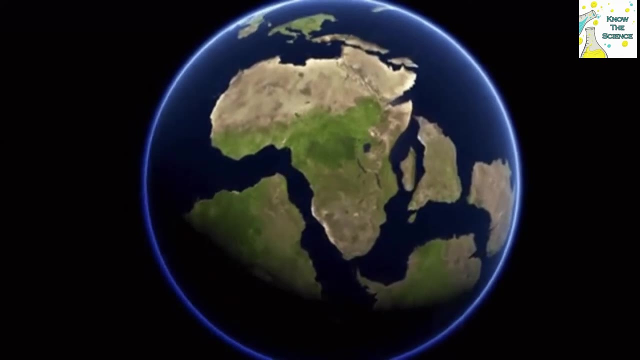 time. Even though humans live on the crust, they do not often feel these movements, as they are very slow and the sheer size of each plate is so large. Nevertheless, these shifts still have great impacts on human life, as the movement of plates is what creates changes in the geographical 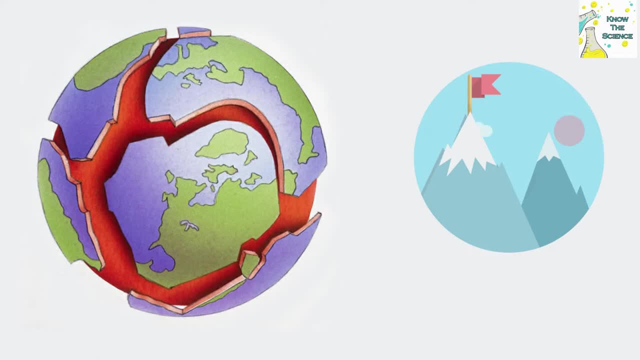 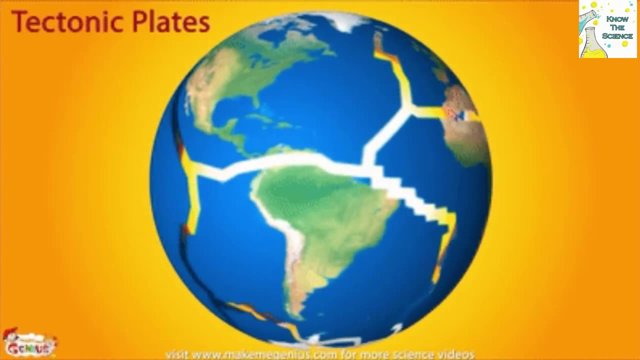 structure of the surface of the Earth. In this way, mountains are created over time. When these plates collide, there is a great deal of mass and pressure, which suddenly comes to a stop, and it is this movement that forces the Earth into buckles or protrusions, which are known. 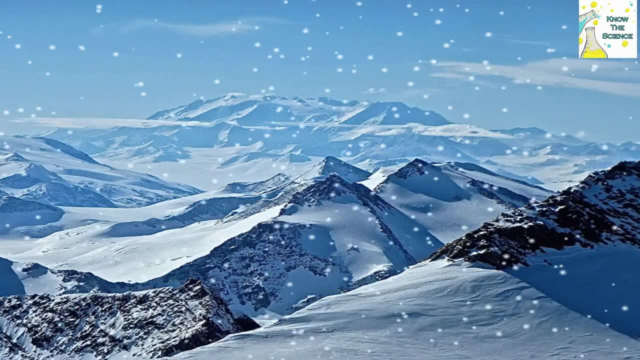 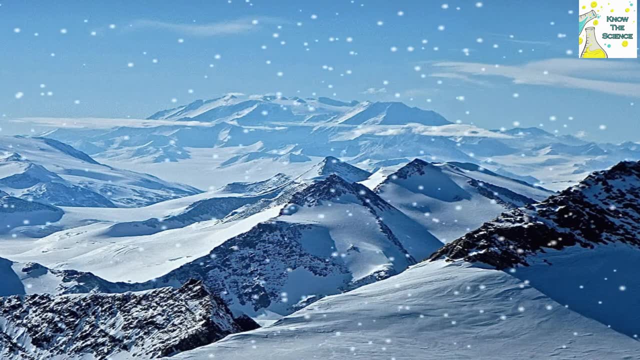 as mountains. Depending on how these plates move, the Earth will move in a certain way. one of three types of mountains can be formed. The three types of mountains or mountain ranges are volcanic, fold and block mountains, each of which is formed in a different way. 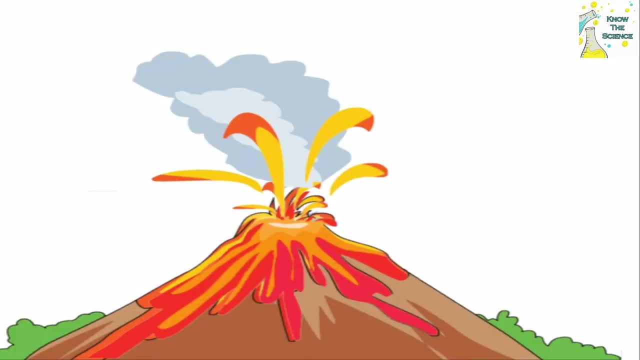 Formation of Volcanic Mountains. Volcanic mountains are formed in areas where there is volcanic activity. This means that there is a place in the Earth's crust where there is a crack or volcanic vent. Magma or molten rock is lighter. 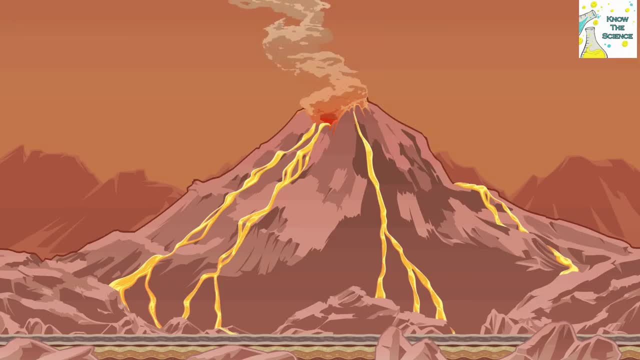 in weight than the solid rock around it. Because of this, it tends to rise to the surface. Similarly, pressure and heat can build up underground and force an eruption of lava out of the volcanic areas. This magma bursts out of the ground and creates lava flows. 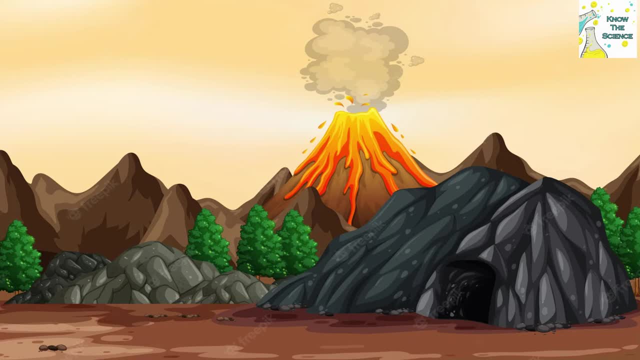 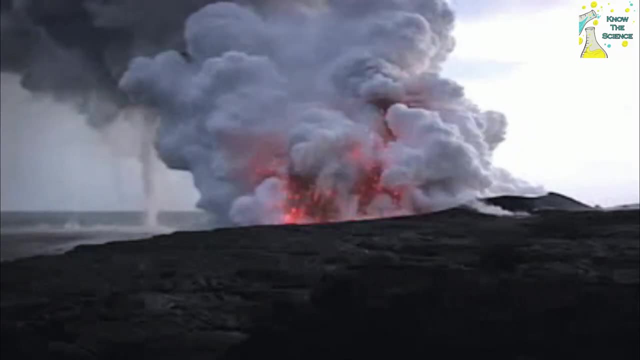 which cool and harden in the open air. Similarly, ash and magma can be ejected high into the air, where they cool and fall to the Earth as debris. Both lava flows and debris build up around the volcano's opening, Creating Volcanic Mountains. 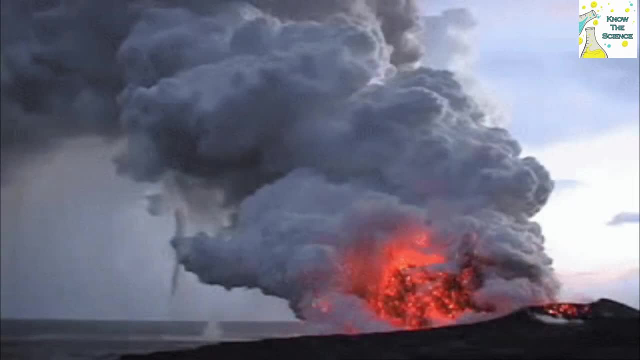 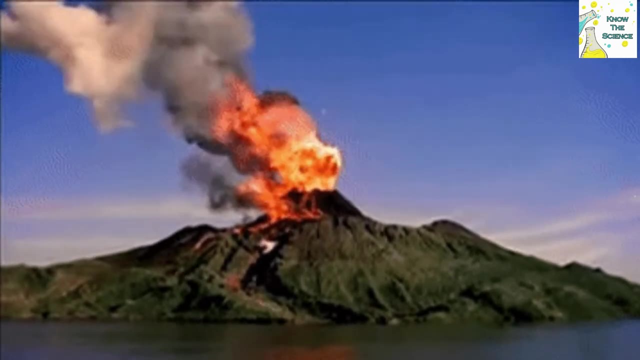 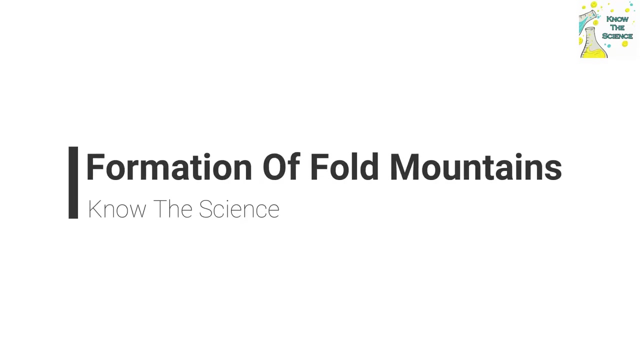 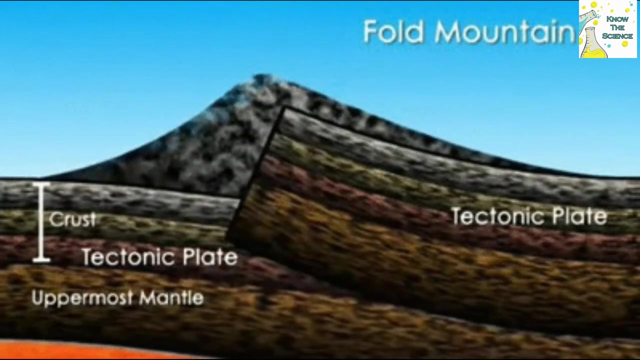 In many cases of larger mountains, this process has happened over centuries, with multiple eruptions slowly building the mountain higher and higher. These two different ways in which volcanoes form mountains are described as cones or shield mountains. Formation of Fold Mountains. Like all mountains, fold-type mountains are created in areas where tectonic plates meet.